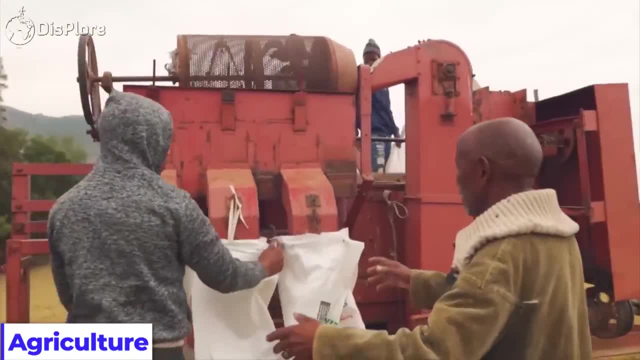 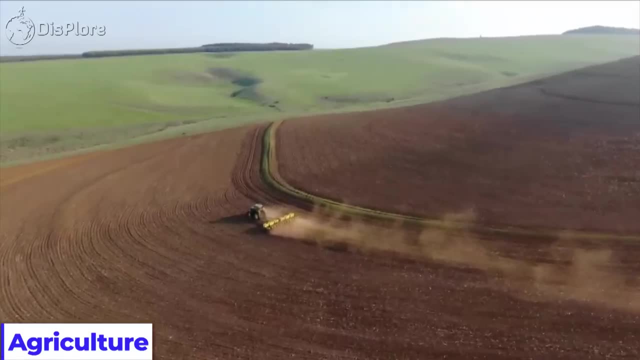 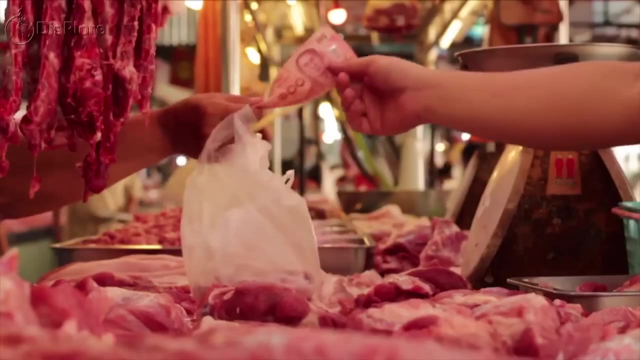 of corporate and private intensive and extensive crop farming systems, including vegetable, fruit, nuts and grain production. The world-developed commercial farming sector in South Africa is the backbone to the country's agricultural economy and, in 2020, showed the best growth rate of all economic sectors, coming in at 13.1%. As a matter of fact, the agricultural sector 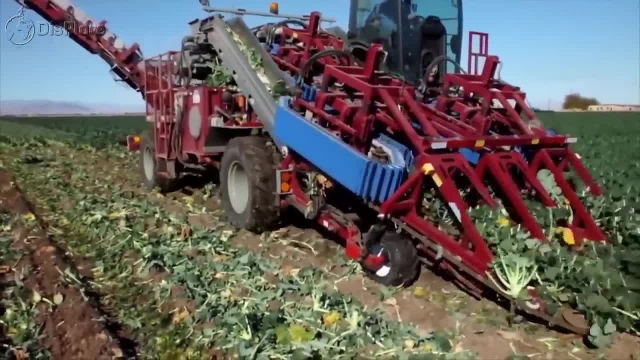 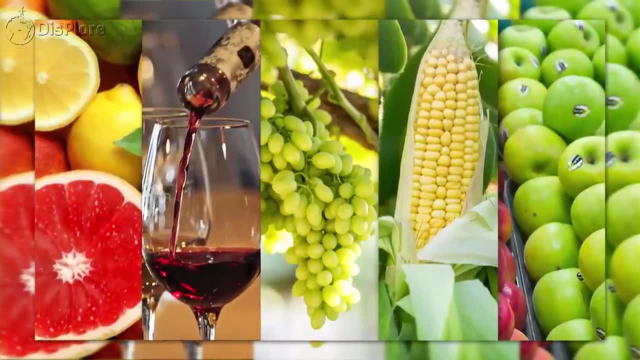 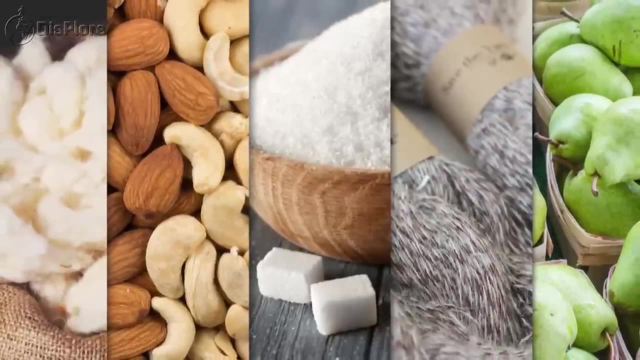 contributed around 10% to South Africa's total export earnings in 2020, at a value of 10.2 billion dollars. Citrus, wine, table grapes, corn and apples accounted for the largest exports by value. South Africa also exports wool, nuts, sugar, mohair and pears, just to name a few. 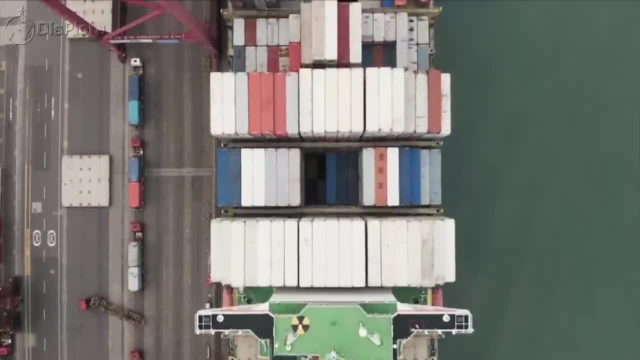 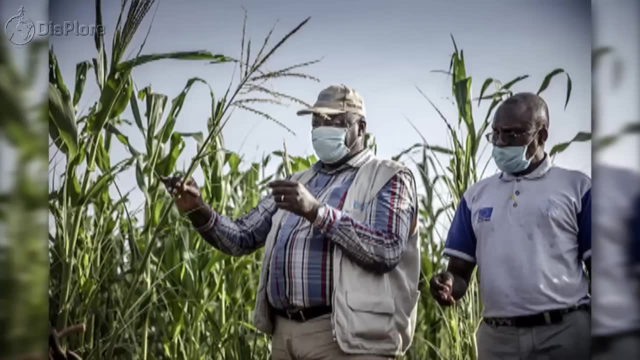 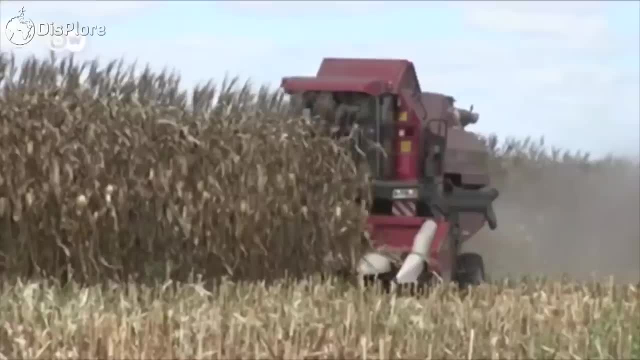 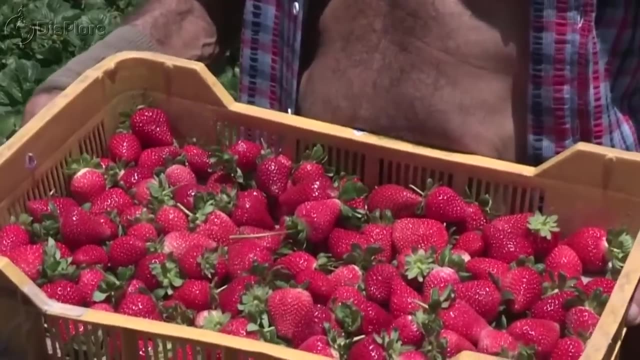 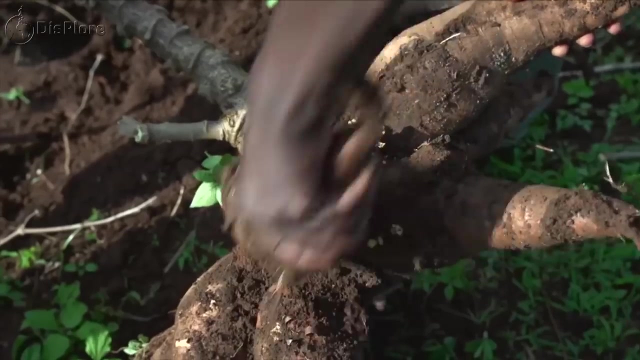 South Africa is emerging from one of the best years. The 2020-2021 season saw bumper harvests for grains, oilseeds and some fruits. These boosted export earnings and improved farm incomes, especially for grains, where the large harvests coincided with higher crop prices. 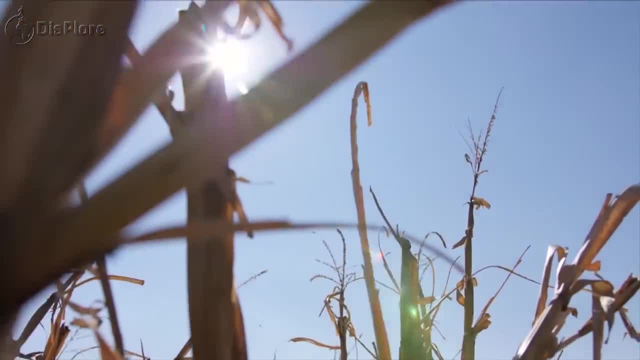 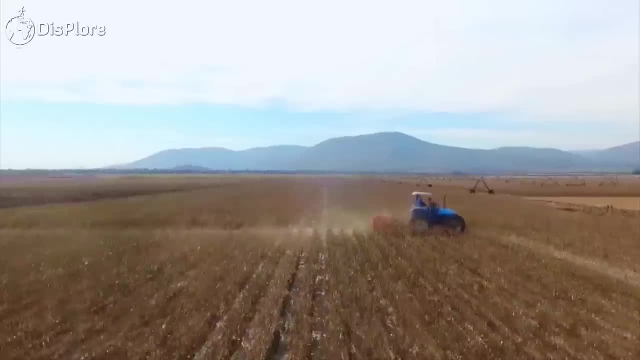 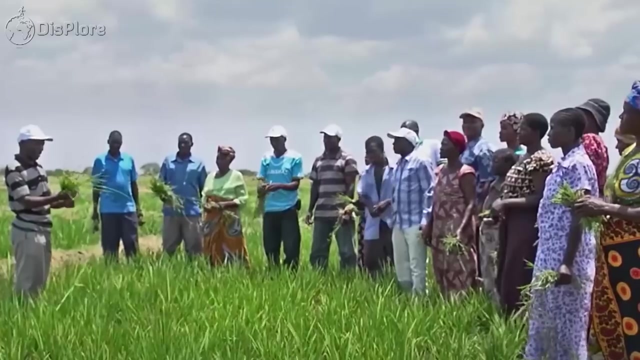 This is thanks to its good climate. The South African climate ranges from tropical to Mediterranean, allowing for a multitude of farming opportunities. The country's biodiversity ensures that products such as grains, fruit and wine are exported and preferred for its exceptional quality. This is a growing demand to improve subsistence farming or informal, small-scale farming in South 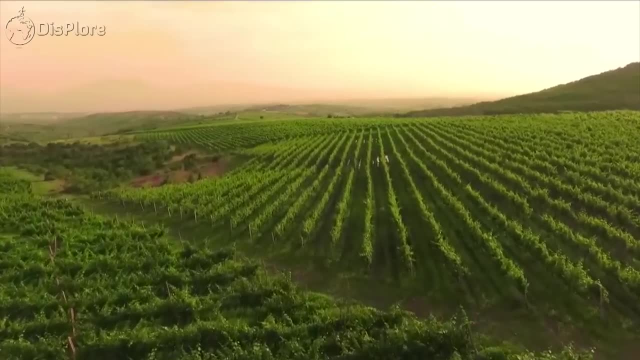 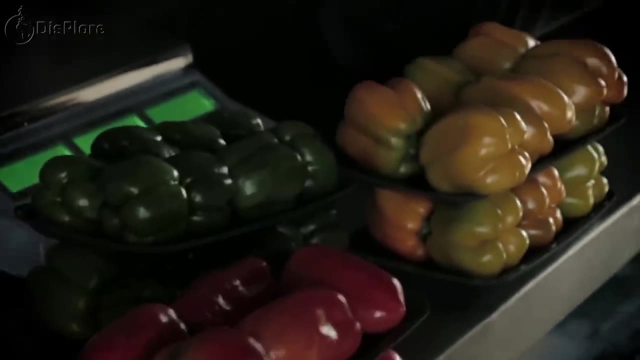 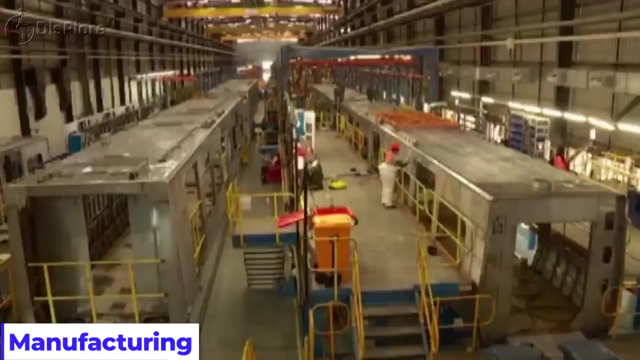 Africa. There are approximately 32,000 commercial farmers in South Africa, of which between 5,000 and 7,000 produce approximately 80% tons of agricultural output. Manufacturing Previously considered the growth engine of the South African economy. the manufacturing in the 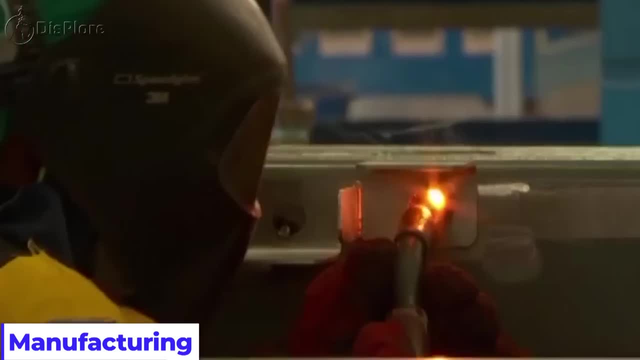 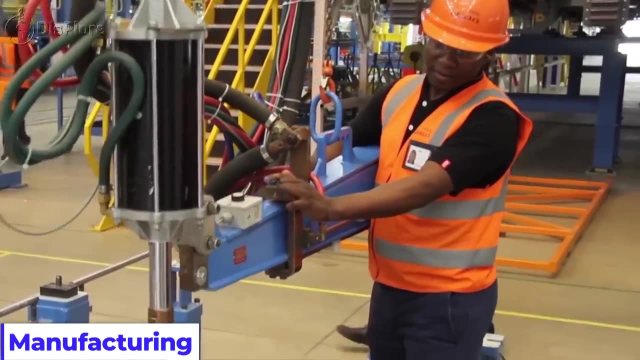 industry has been in decline, with local manufacturers facing multiple challenges. The manufacturing sector has been an area of focus for government, as it offers the greatest potential for job creation and economic growth. In 2016,, the government launched the Black Industrialist scheme. 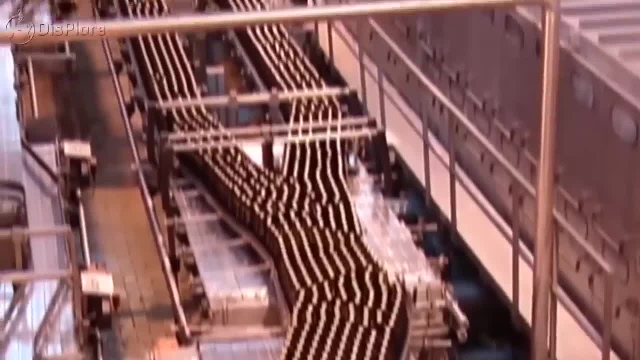 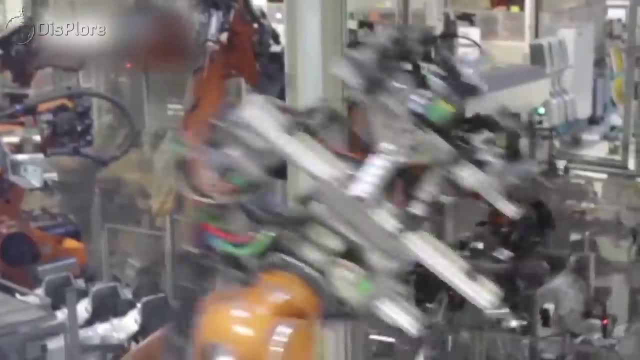 which has the manufacturing sector as a key focus to help stimulate the manufacturing industry. To date, the scheme has backed 102 industrialists, including some success stories in the manufacturing sector, such as micro-industries and industrial production. The manufacturing industry has been 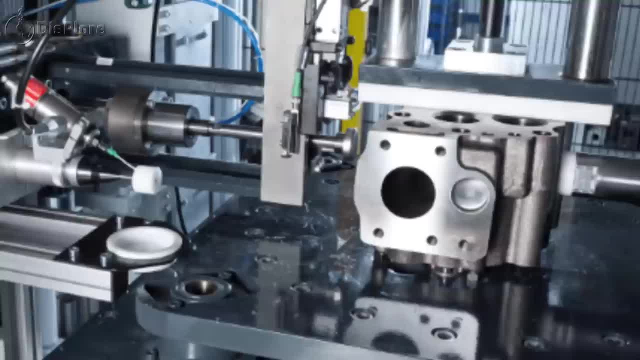 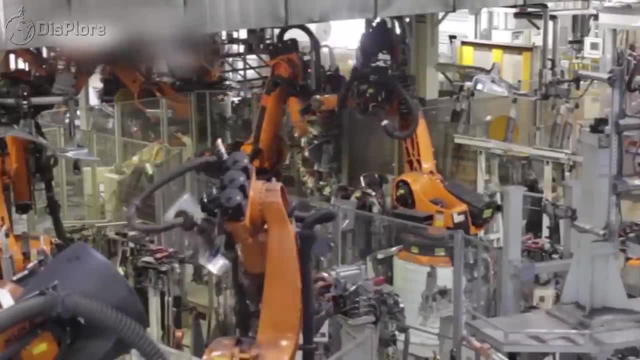 in decline, as it offers the greatest potential for job creation and economic growth: Automotive in KwaZulu-Natal, which manufactures and supplies valve guides and valve seats to original vehicle manufacturers and aftermarket service providers. Minelli Pets, an agro-processing company. 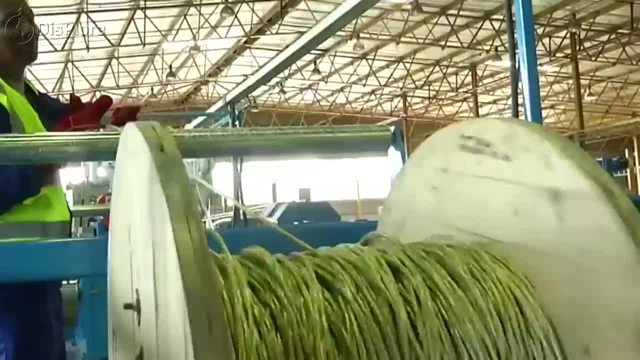 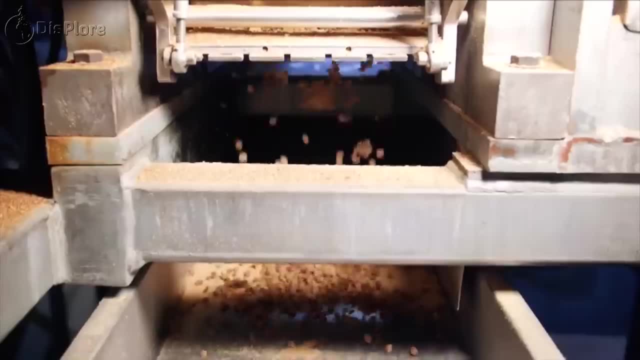 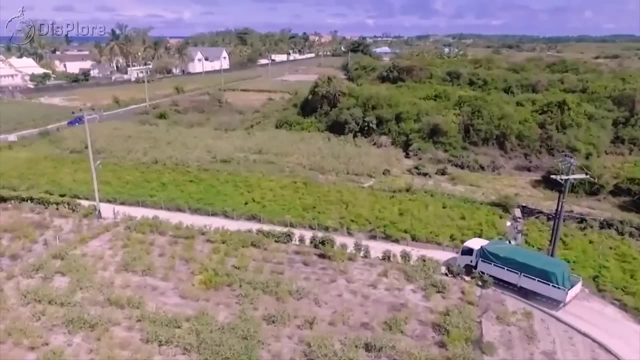 which produces high-end pet food. United Industrial Cables, which receives millions for the manufacturing of a variety of copper cables. Nevertheless, the major manufacturing sectors are food processing and the production of textiles, metals and chemicals. Agriculture, fisheries, provide the basis for substantial activity in wheat, fish and fruit canning. 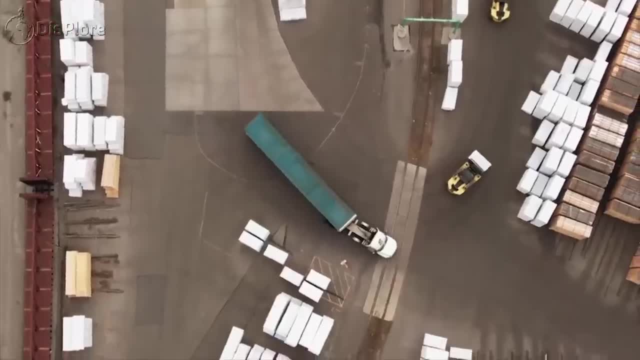 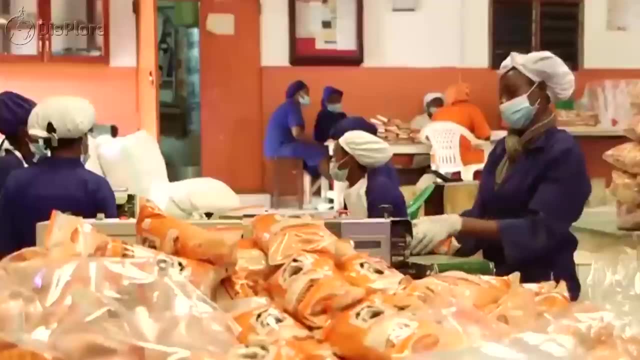 sugar refining and other processing. More than half these products are exported. However, in January 2022, manufacturing production output increased by 2.9%, compared to a 0.2% fall in December 2021.. The rate of growth in January was the fastest since June. 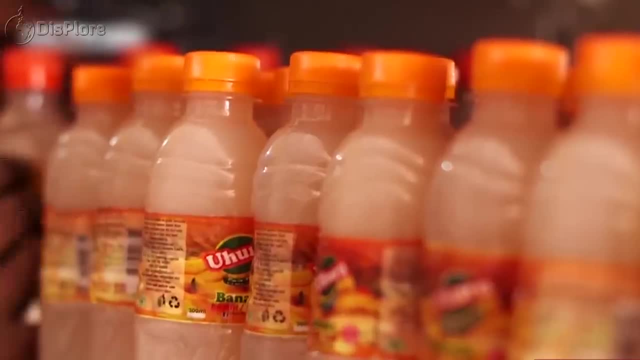 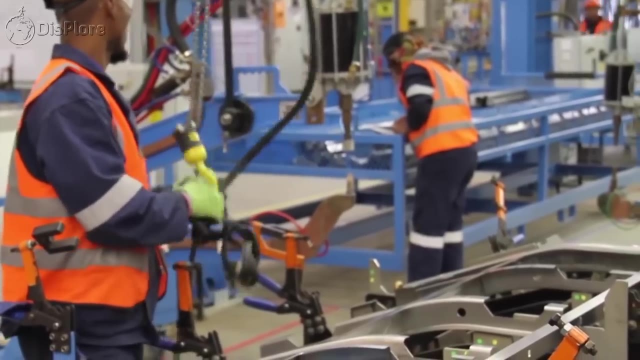 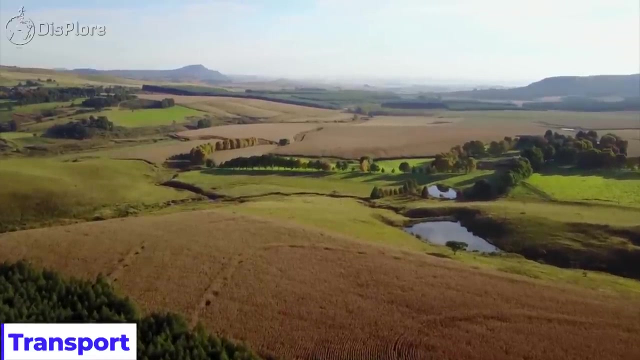 2021.. Rebounding activity in the food and beverage, basic iron and steel, non-ferrous metal products, goods and equipment sub-sectors contributed significantly to the improvement. Transport South Africa contains no navigable rivers. Coastal shipping provides the only water transport. 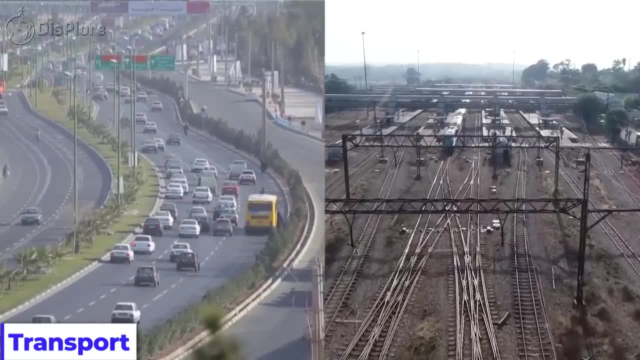 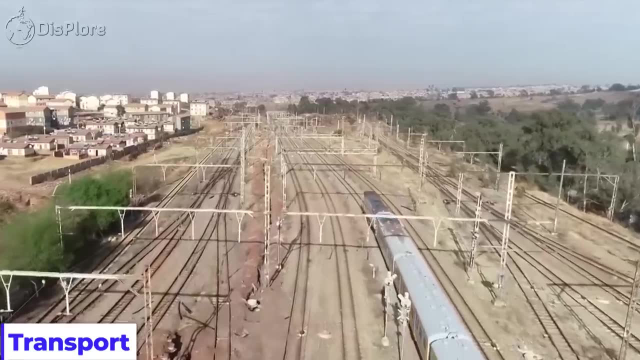 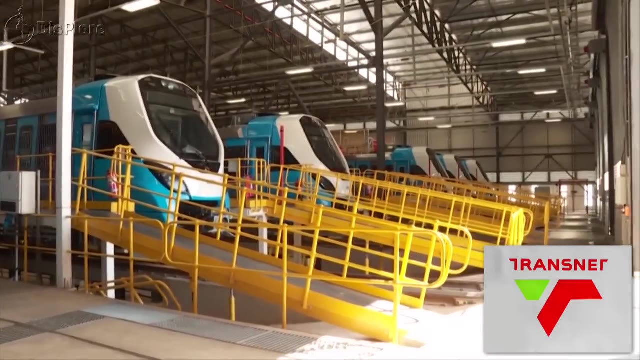 The country's network of roads and railways, the most extensive in Africa, handles most of the transportation demand, supplemented by air travel. The railway system, which serves all the major cities, smaller towns and many rural areas, is almost entirely owned and operated through the transnet public corporation, although parts of transnet are gradually being 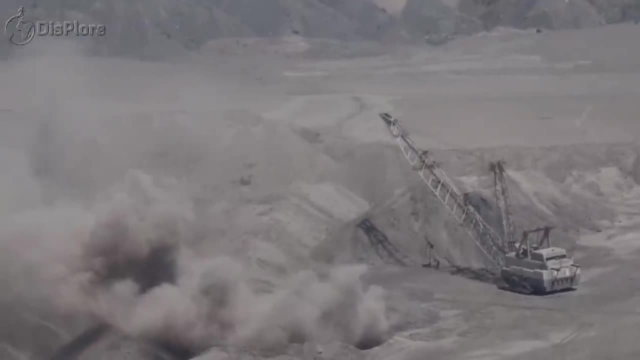 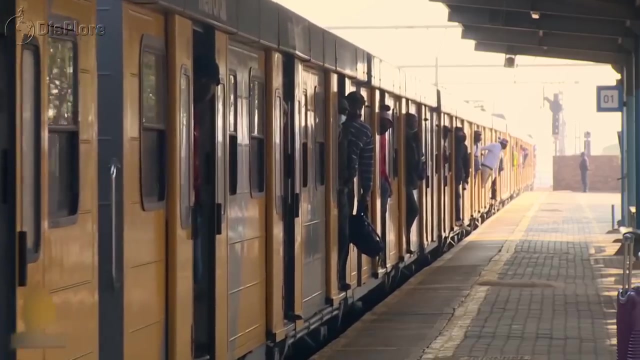 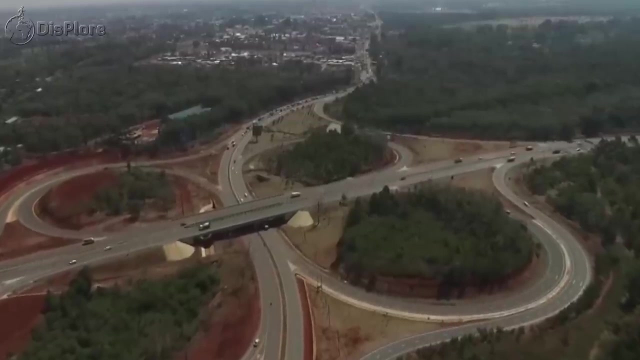 privatized. Coal and iron ore, among other products, are transported on these lines. Long distance passenger services have declined, but many commuters use train services in all the major urban centers. The road network, on the other hand, contains some 185,000 miles of roads. 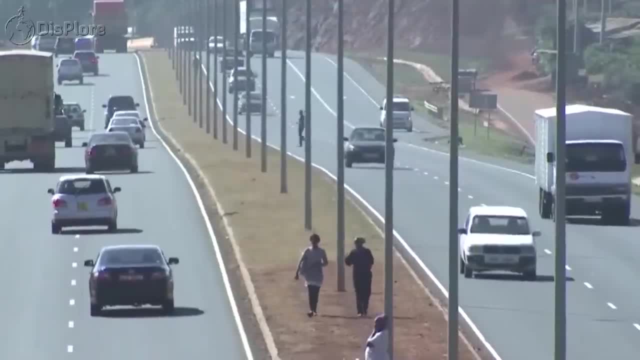 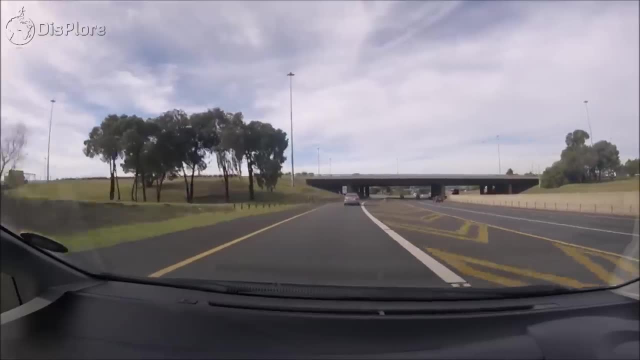 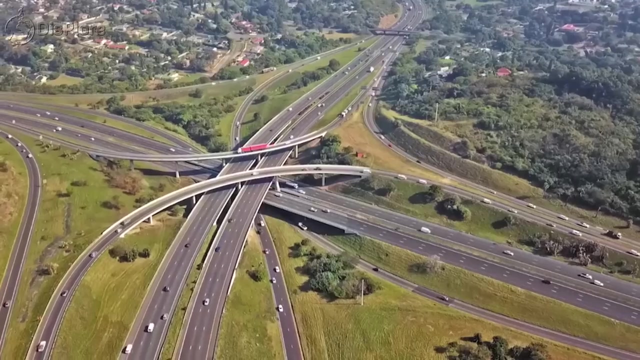 ranging from rural unpaved stretches to multi-lane freeways. About two feet of the roads are paved. Locked se SNIT据. Most towns are connected by two-lane highways. multi-lane freeway systems extend around the four major urban areas, but over long distances only Johannesburg and Durban are connected. 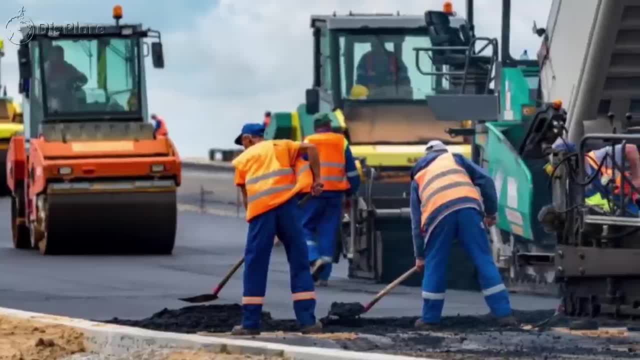 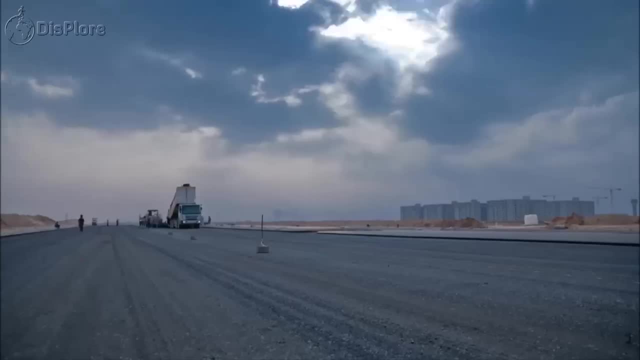 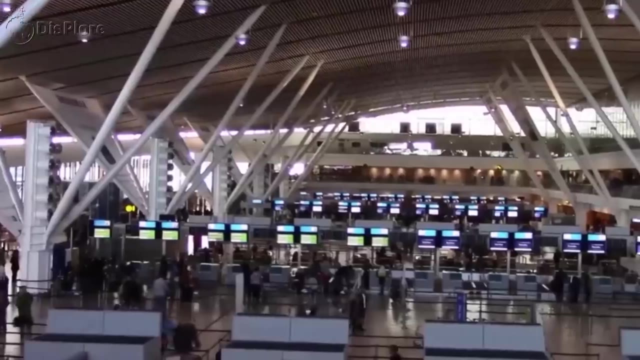 by such a highway. However, most of the responsibility for maintaining and regulating roads fall to the different levels of government, but some long-distance roads have been transferred to the private sector and transformed into toll roads. Meanwhile, in inland air services, both passenger and freight are operated by the state-owned South African Airways and by an increasing number of private competitors. Air services connect all major cities. South African Airways and many foreign carriers fly between South Africa and all neighboring countries. International service extends worldwide. The OR Tambo International Airport near Johannesburg is the main hub of the country's airport. 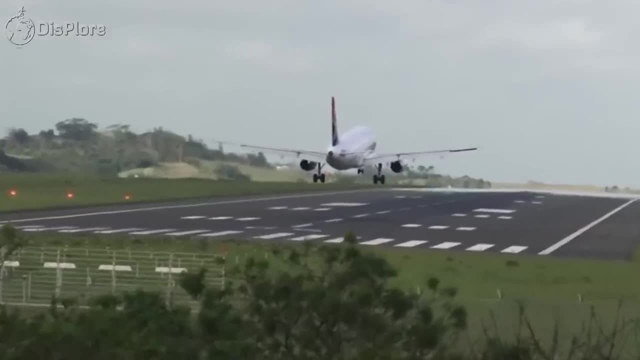 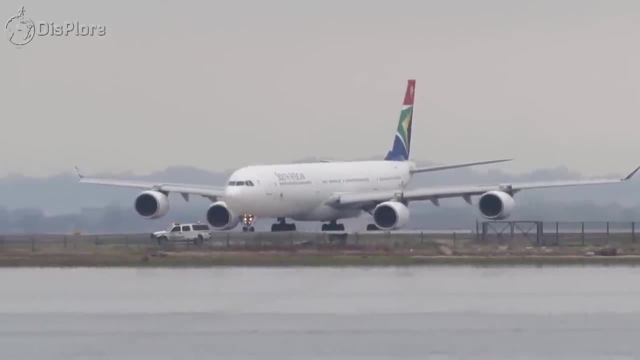 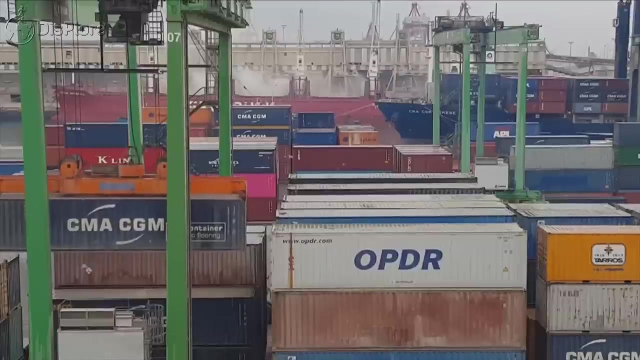 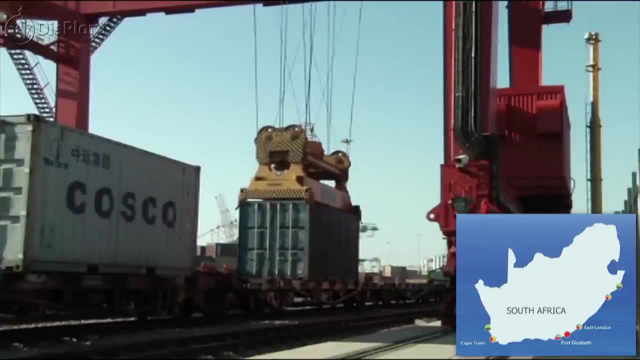 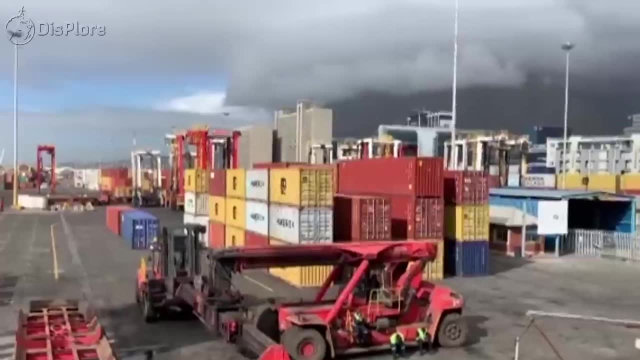 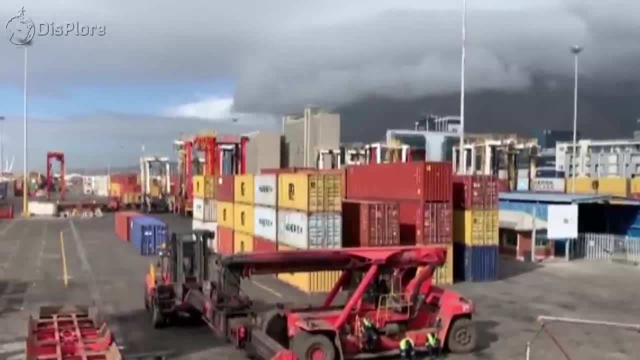 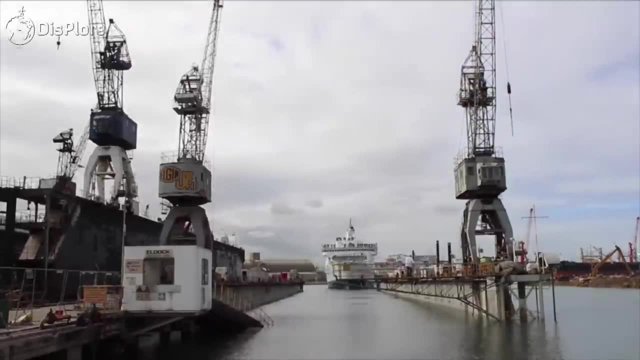 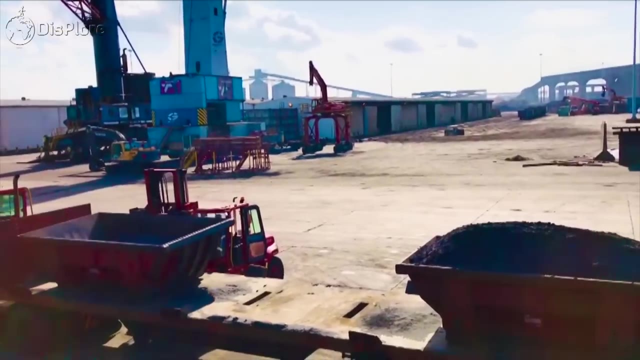 Zimbabwe, Zambia and the Democratic Republic of the Congo. Maputo, the port closest to Johannesburg, serves many areas of the northern provinces. Newer ports have also been developed at such places as Richards Bay, which handles exports of coal, on the north coast of KwaZulu-Natal and in the excellent natural harbors of the 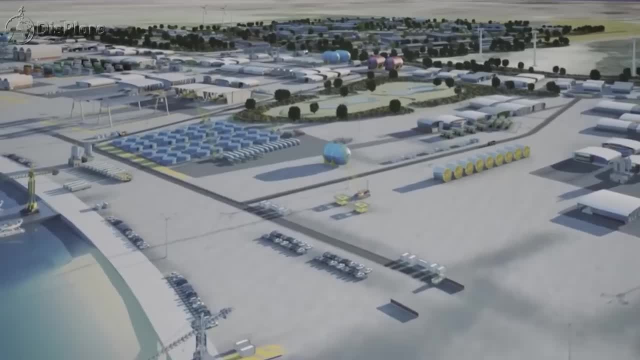 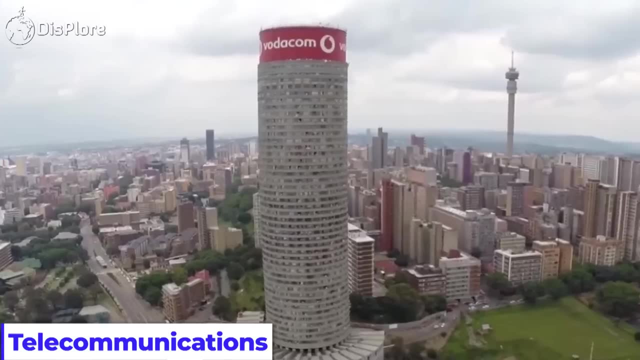 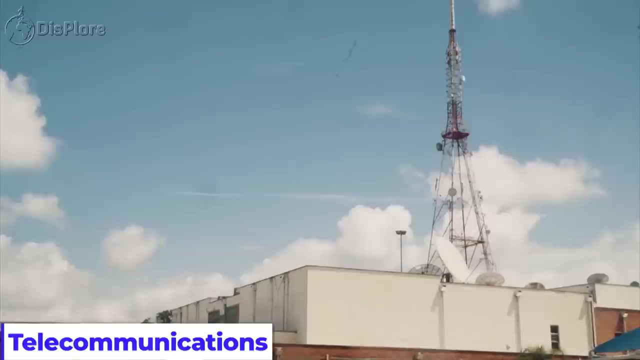 city of Hannahsburg harbour at Saldana Bay, north of Cape Town, from which iron ore is exported. Telecommunications: Telecommunications infrastructure in South Africa provides modern and efficient service to both urban and rural locations. This includes everything from 5G to Gigabyte broadband in terms of cellular and internet. 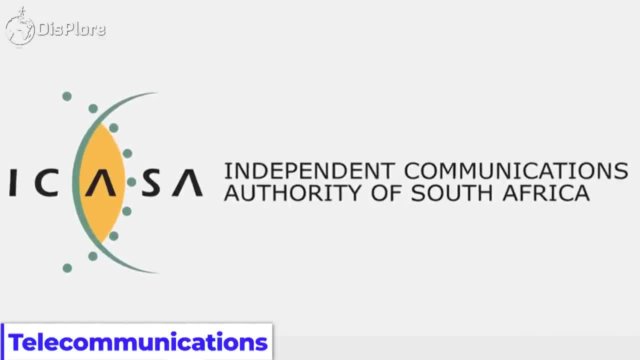 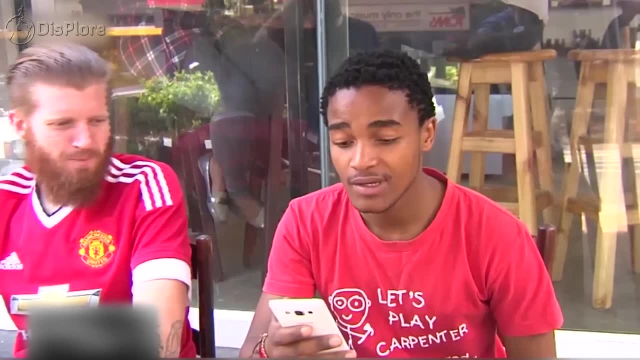 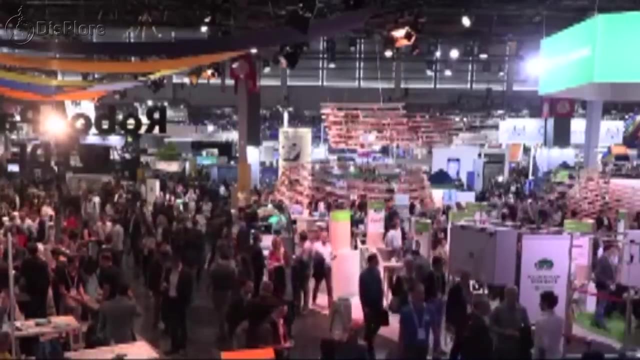 services. The Independent Communications Authority of South Africa is the watchdog of the telecommunications in the country. Five mobile phone providers in South Africa are responsible for delivering mobile services to over 50 million subscribers, and the country is regarded as having the world's fourth most advanced mobile telecommunications network. 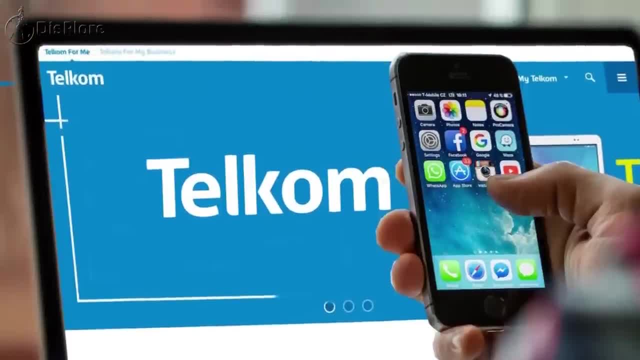 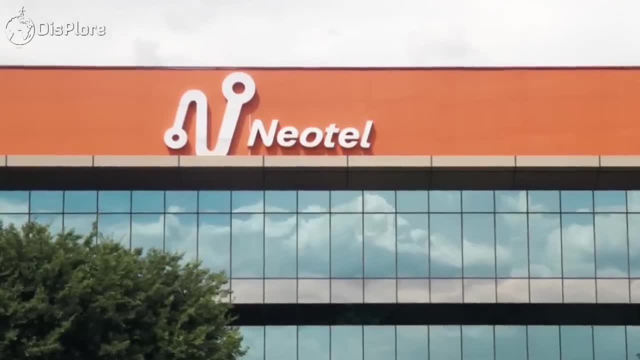 Vodacom, MTN, Cell-C, Telcom Mobile and Rain are the five primary cellular providers, with Liquid Telecom's Neotel no longer providing mobile services. However, Vodacom and MTN controls about 75% of the country's mobile telecommunications. 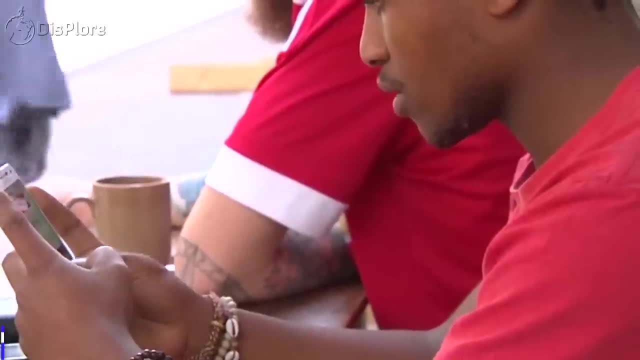 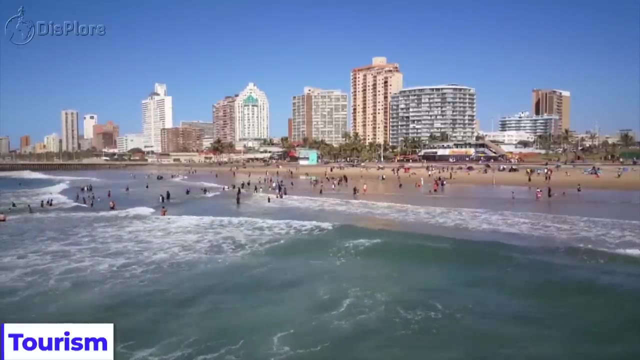 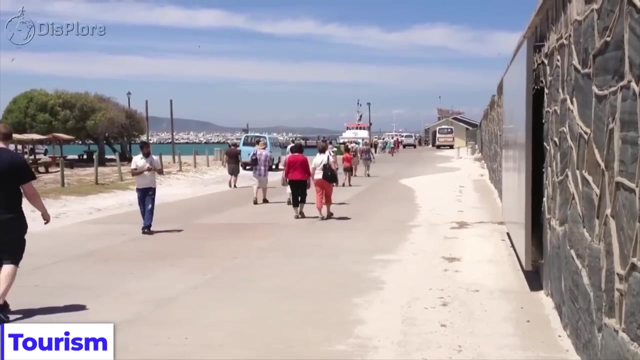 services in South Africa Tourism. South Africa is a popular tourist destination with around 860,000 arrivals per month, of which around 210,000 come from outside the African continent. The industry accounts for a substantial amount of the country's revenue. 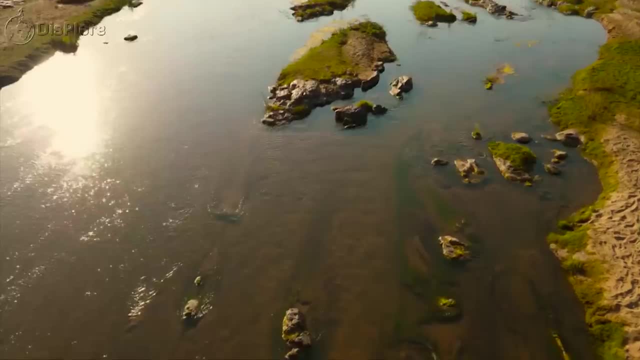 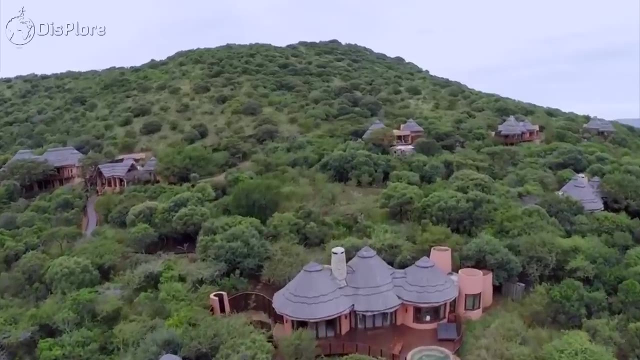 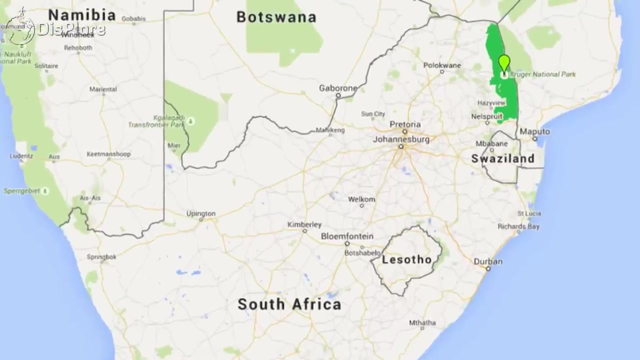 South Africa offers both domestic and international tourists a wide variety of options, among others, the picturesque natural landscape and game reserves. Some of the most popular destinations include several national parks, such as the expansive Krugu National Park in the north of the country, the coastlines and beaches of the KwaZulu-Natal. and Western Cape Provinces and the major cities like Cape Town, Johannesburg and Durban. The country is also particularly rich in plant diversity, with a wide variety of biomes found across the country. This includes the grasslands in the high valleys of the KwaZulu-Natal and western Cape Provinces. 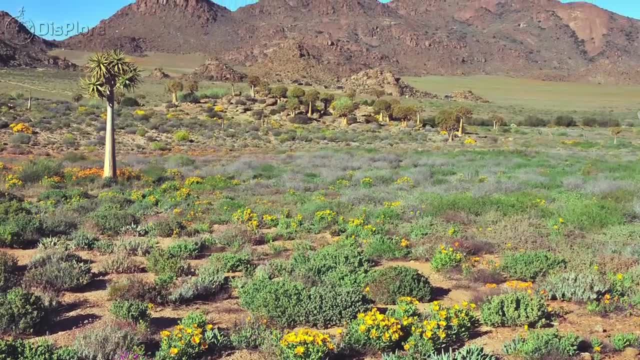 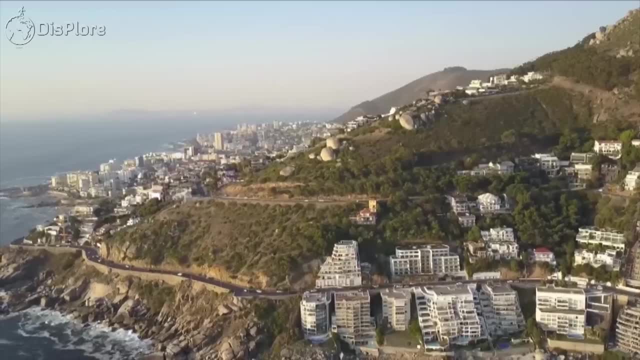 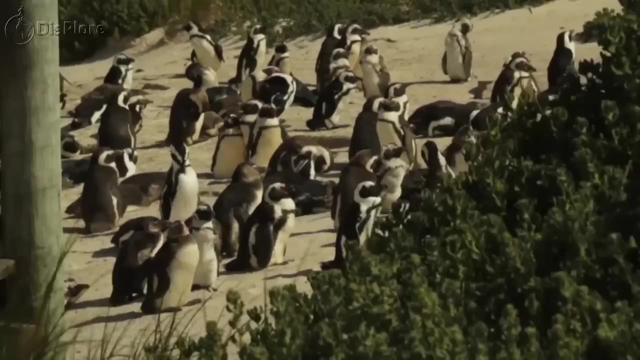 the high veld, the succulent karo in central South Africa and the endemic fin bones biome, constituting the majority of the area and plants live in the Cape Floristic region of the Western Cape. This rare vegetation is protected as part of the Table Mountain National Park, which 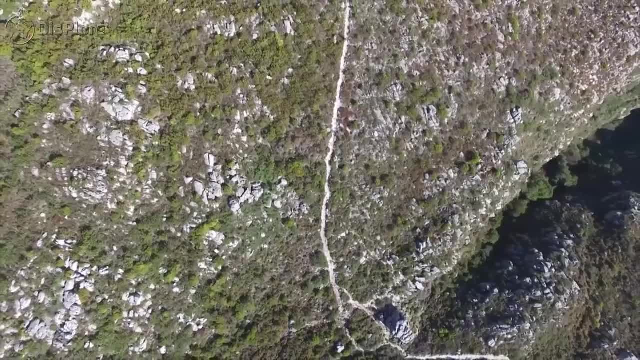 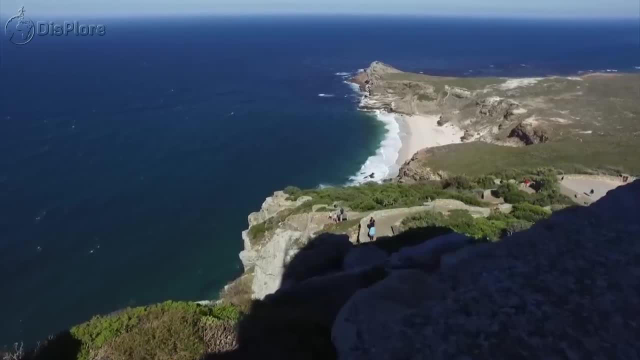 was the most visited national park in South Africa between 2014 and 2015,, with a total of 2,677,767 visitors. The top five of the top five national parks in South Africa are the National Park of the World, the National Park of the World and the National Park of the World. 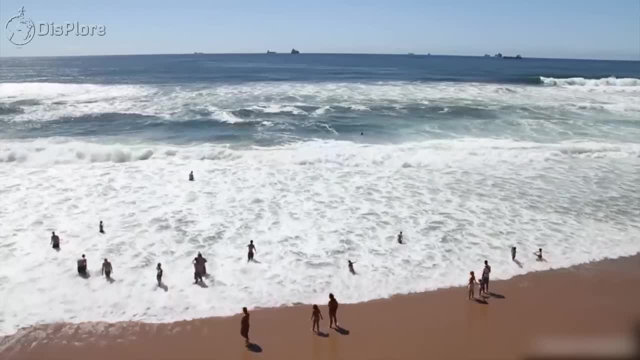 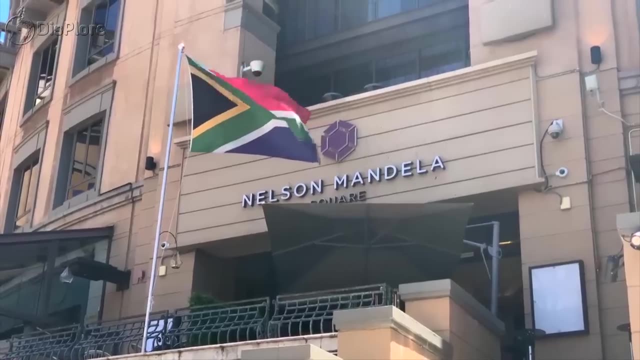 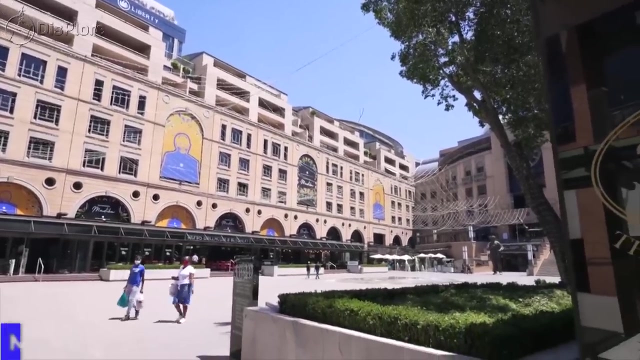 The top five overseas countries with the largest number of tourists visiting South Africa are the USA, the UK, Germany, the Netherlands and France. Most of the tourists arriving in South Africa from elsewhere in Africa come from the SADC countries. Mining Mining has always been a major industry in South Africa In 2013,, diamond and gold production were significantly below their peaks, yet South Africa remained the world's fifth-largest gold producer. The world's largest gold producer is the United States. The United States is the world's largest gold producer and a geological treasure trove. 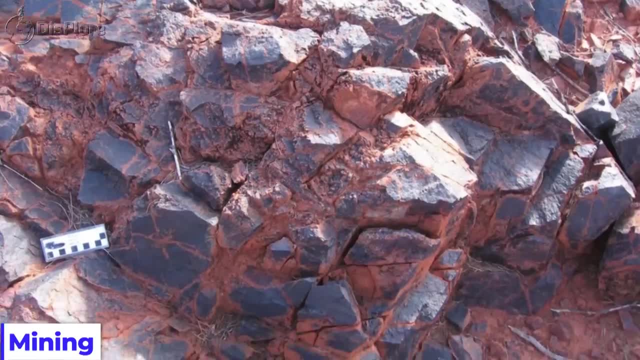 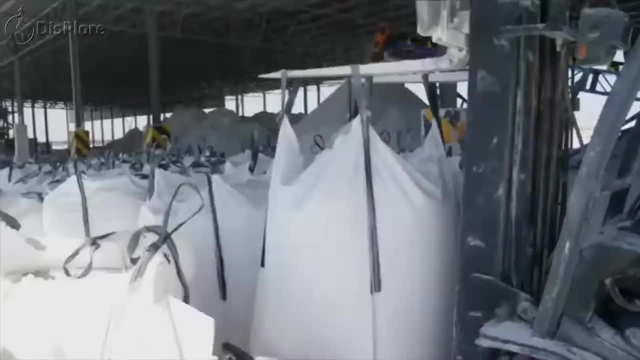 It produces the most chrome, manganese, platinum, vanadium and vermiculite in the world. It is the second-largest producer of elemanite, palladium, rutile and zirconium. It is also the world's third-largest coal exporter. 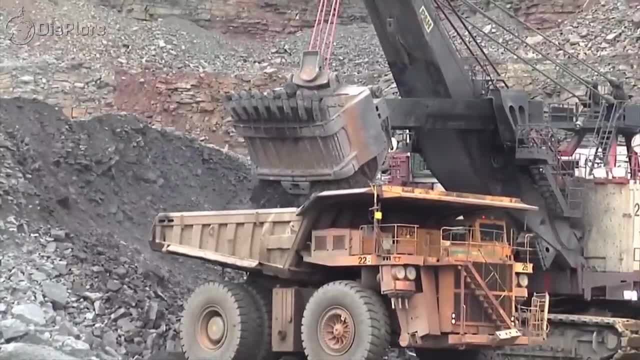 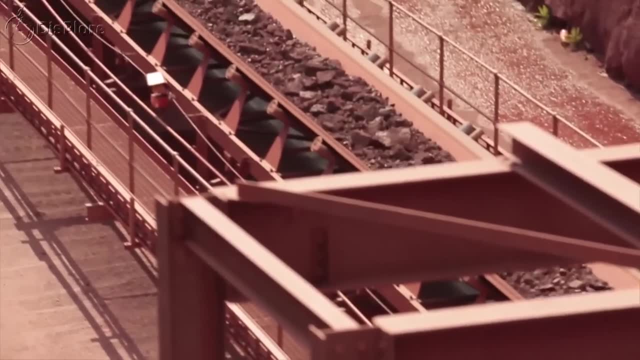 South Africa is also a huge producer of iron ore. In the year 2012,, it overtook India to become the world's third-biggest iron ore supplier to China, The world's largest consumer of iron ore. It got its name from gardeau, which octvens coal and steel into uranium ore to serve igual. 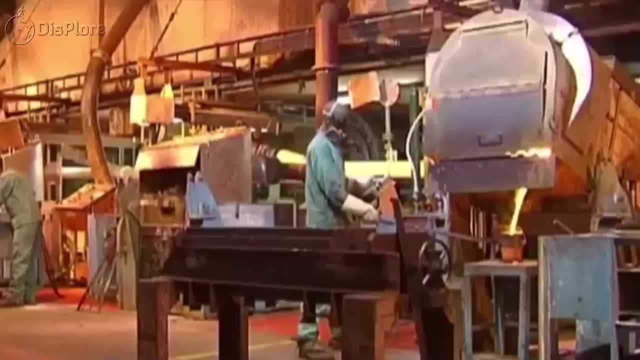 use in the world, When Gorging and incinerating uranium ore was 아� all. it's only a matter of time before the world's teeming opinion had a sound revolution. debut is teeming with global revolution, Guer Larsenер. 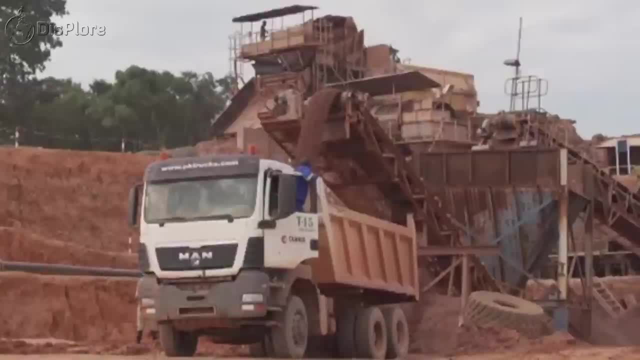 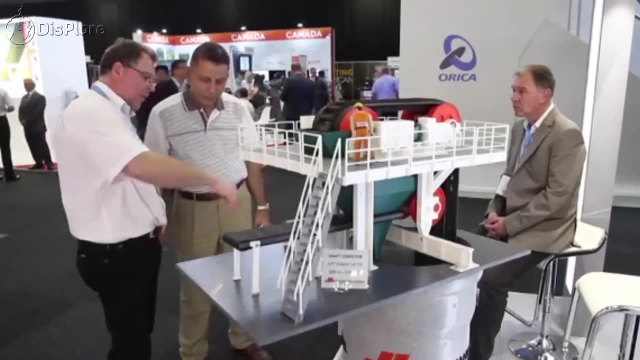 The world's largestinhos gold receptorénergie crimes and thetightening longer supply chains force governmentㅠ The world's largest mining and technologyЕН Le. Coming back to mining, miningBon answered plante parliamentary questions about how to manage actual mining, mining etc. withfer baptism and life, and how to id quicker and. 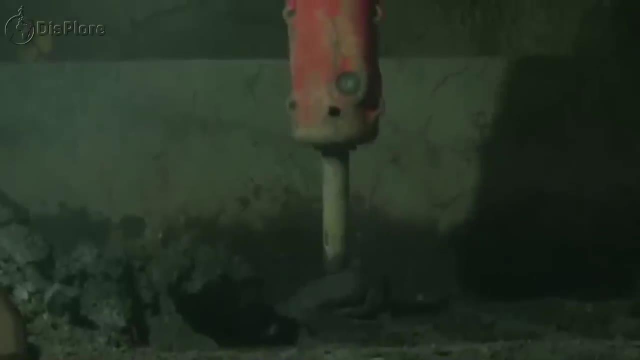 evenly. The habformation is one of the most important اcortex, probably one of China's more legile, long-lasting mining encroachments. 19 years and 21 years ahead In present, we've been to steel-fired coal mines in the World's largest tomatoなんです. 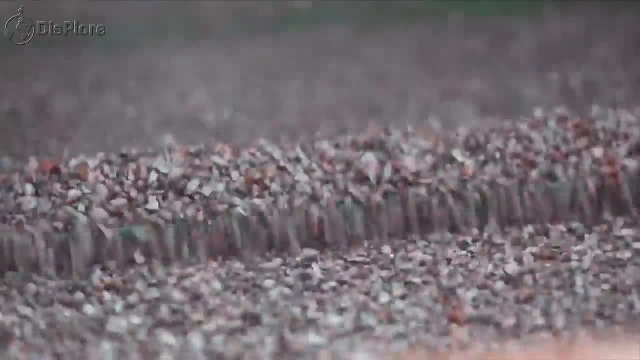 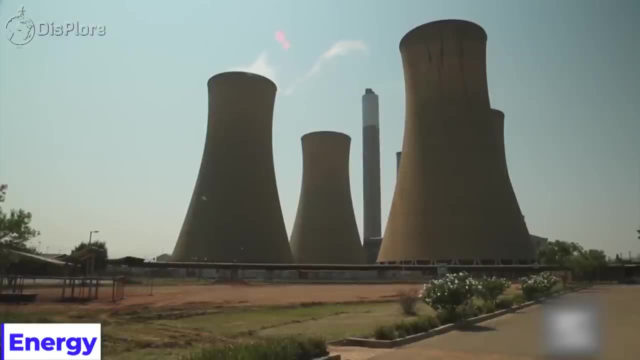 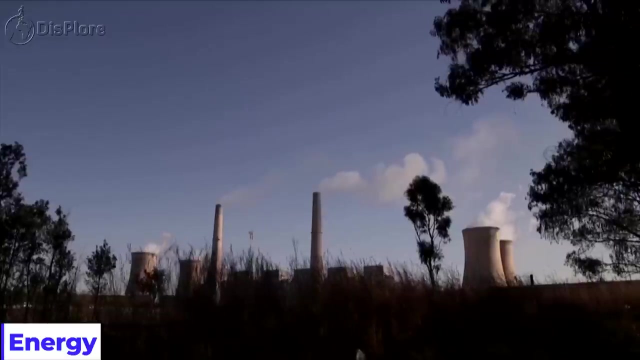 than $2.5 trillion, with 16 commodities ranked in the top 10 internationally. Energy: Nearly all of South Africa's electricity is produced thermally, almost entirely from coal. Most electric power is generated by ESCOM at huge stations in Pumalanga. 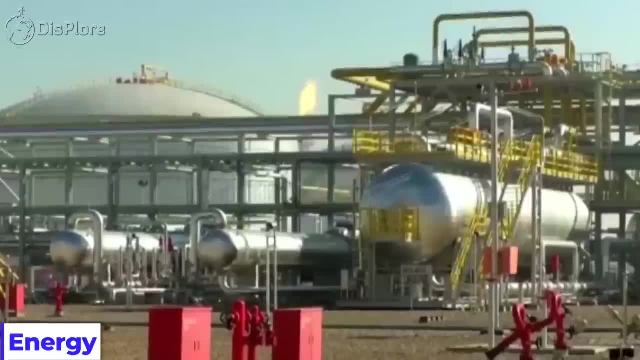 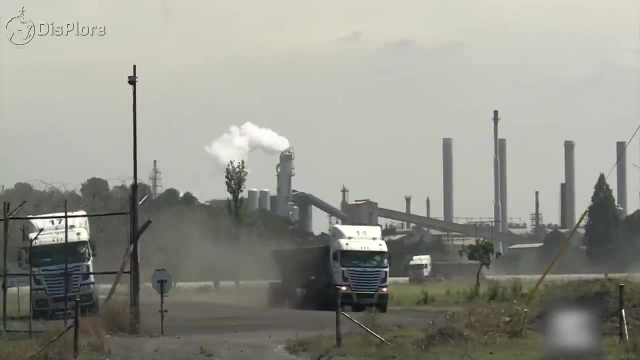 Synthetic coal fuel, as well as imported oil refined at ports or piped to a big inland refinery at Sazoburg, meet a tiny percentage of the country's energy demands. According to the Ministry of Mineral Resources and Energy, South Africa's total domestic 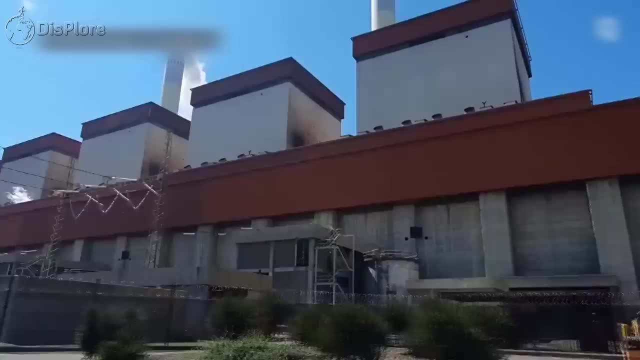 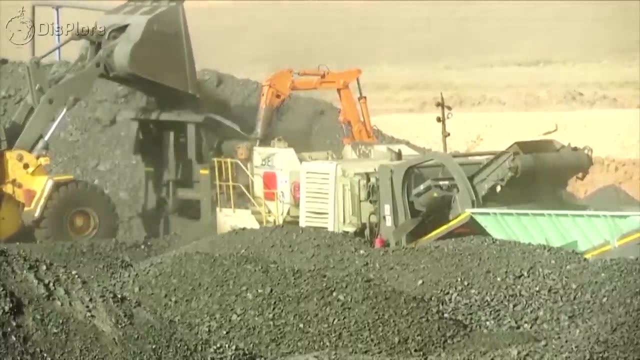 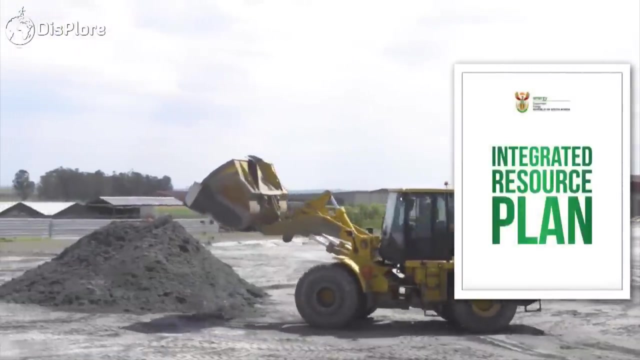 electricity generation capacity is 58,095 megawatts from all sources. Currently, coal is by far the major energy source for South Africa, comprising around 80% of the country's energy mix. However, according to the 2019 Integrated Resource Plan, 24,100 megawatts of. 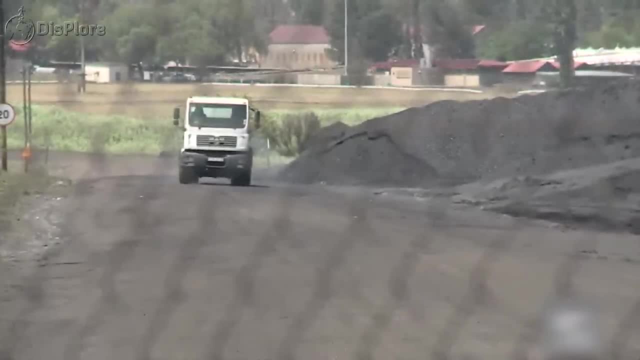 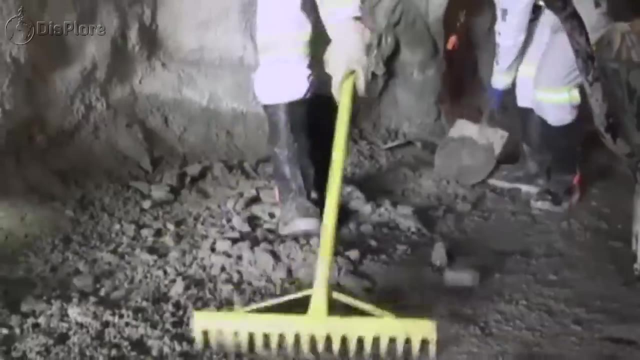 conventional thermal power sources, specifically coal, are likely to be decommissioned within the next 10 to 30 years. While coal may be the dominant source now, its share of total capacity is likely to decrease as more renewable generation comes online in the coming years. 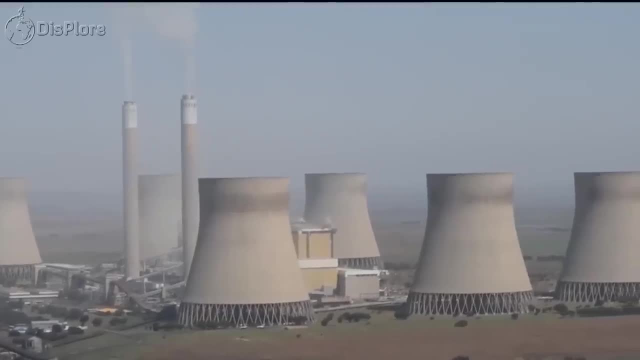 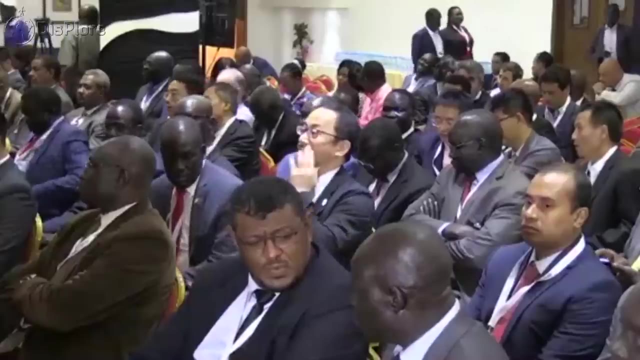 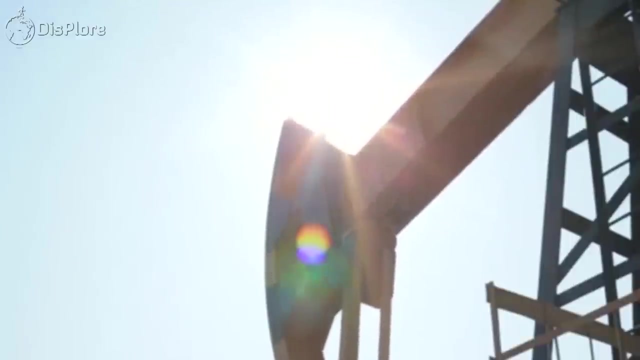 South Africa's Renewable Energy Independent Power Producer Procurement Program for Utility Scale Transactions signed 27 power purchase agreements in June 2018.. The updated IRP outlined a number of steps the government will undertake to improve South Africa's unreliable and deteriorating energy sector, focusing on greater use of natural gas. maintaining the nuclear sector. 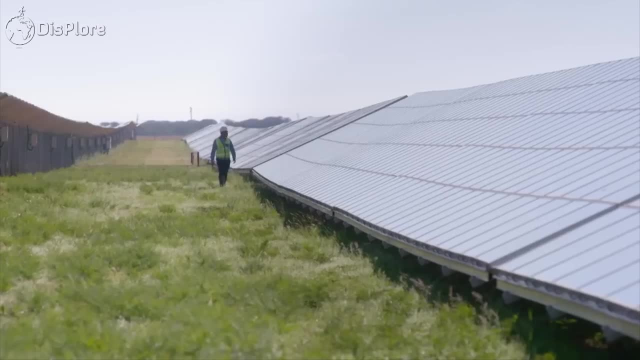 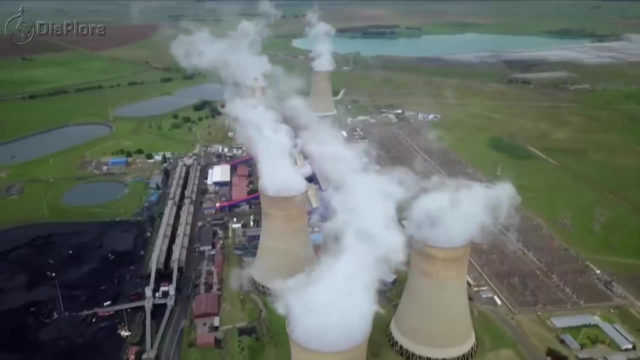 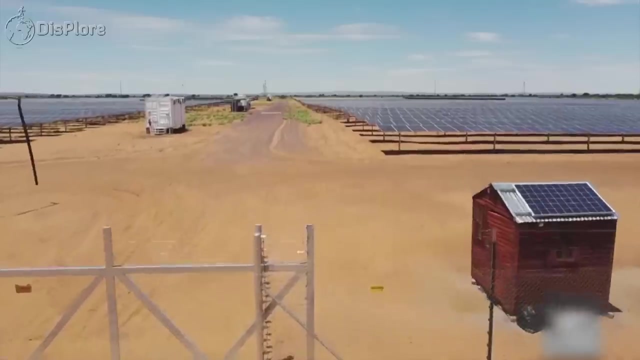 while increasing the focus on social inclusion and a just transition plan to renewable energy. More to it, the country aims to decommission 34 gigawatts of coal-fired power capacity by 2050.. It also aims to build at least 20 gigawatts of renewable power generation capacity by. 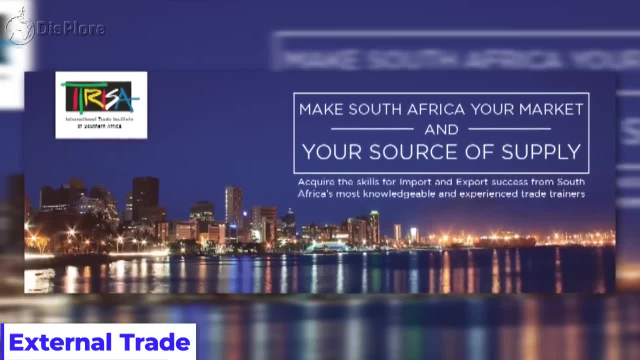 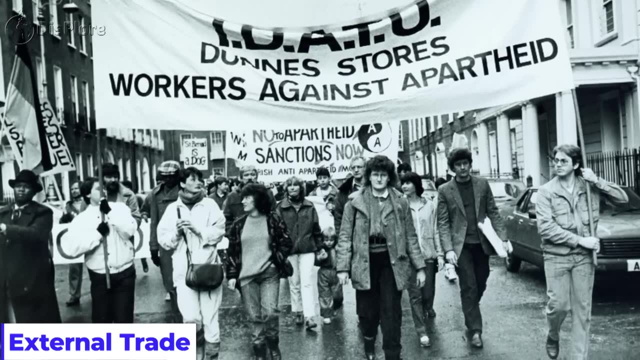 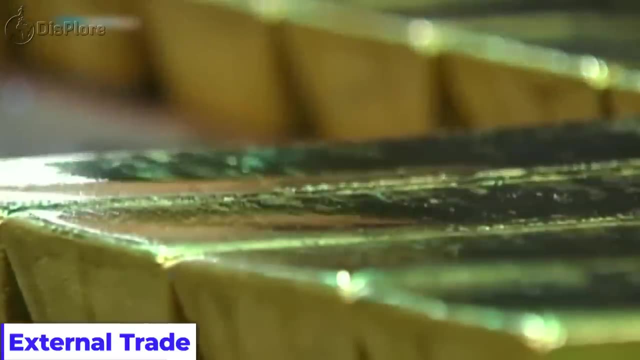 2030.. External Trade: Since the end of apartheid, foreign trade in South Africa has increased following the lifting of several sanctions and boycotts which were imposed as a means of ending apartheid. South Africa is the second largest producer of gold and is the world's largest producer. 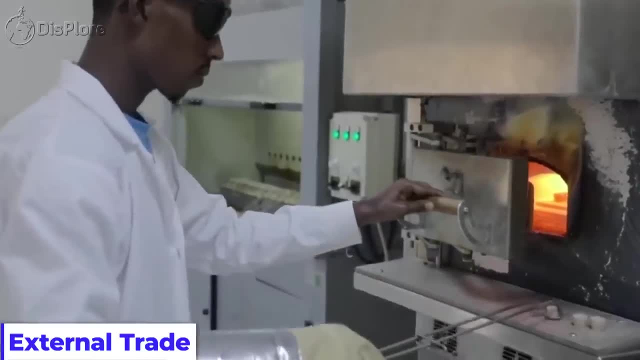 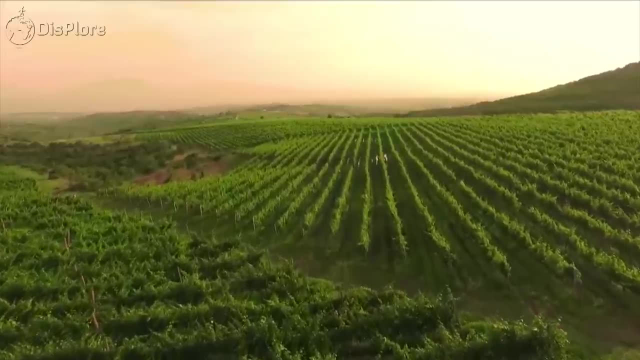 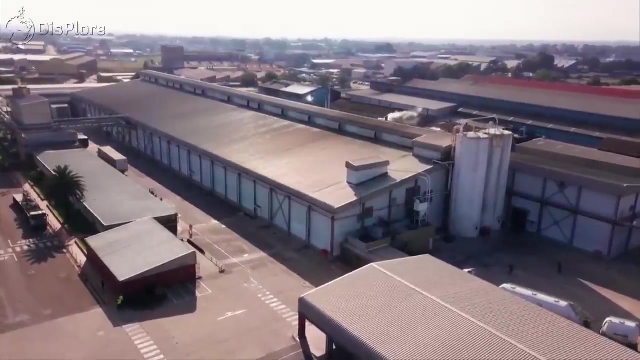 of chrome, manganese, platinum, vanadium and vermiculite. It is also the world's third-largest coal exporter. South Africa also has a large agricultural sector. It is a net exporter of farming products. Imports to South Africa edged up by 0.3% to over $8.7 billion in January 2022, as higher. 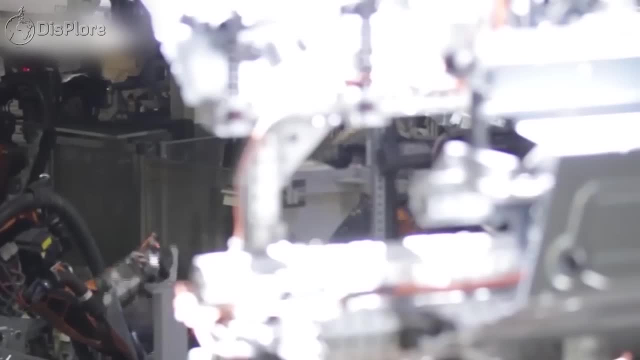 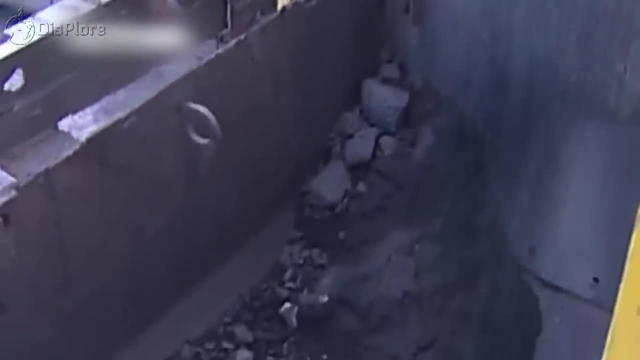 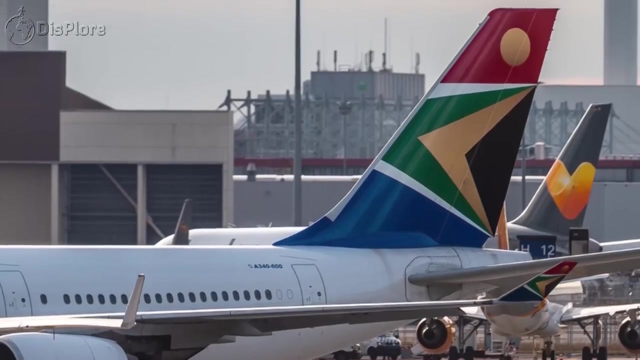 purchases of wood, pulp and paper, original equipment, components and vehicle and transport equipment outweigh decreases in those of mineral products and base metals. South Africa's main imports are machinery, mineral products, vehicles and aircraft vessels, while its main imports are oil and gas. 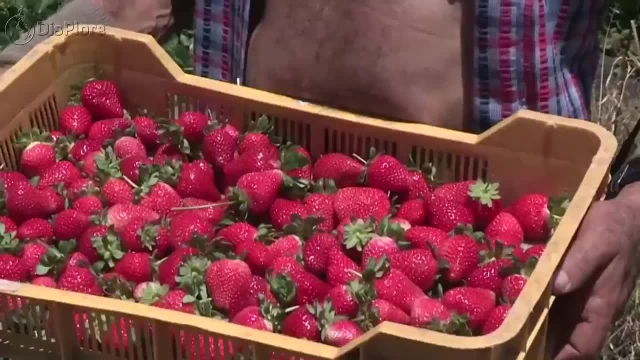 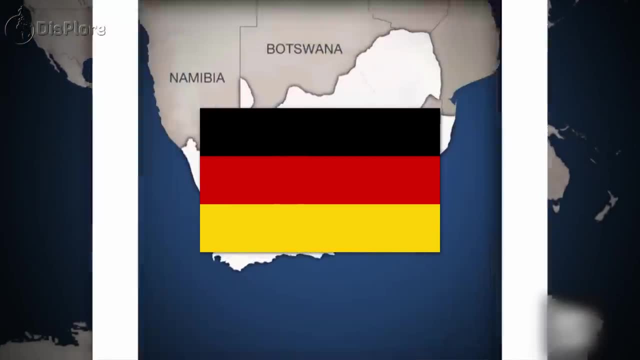 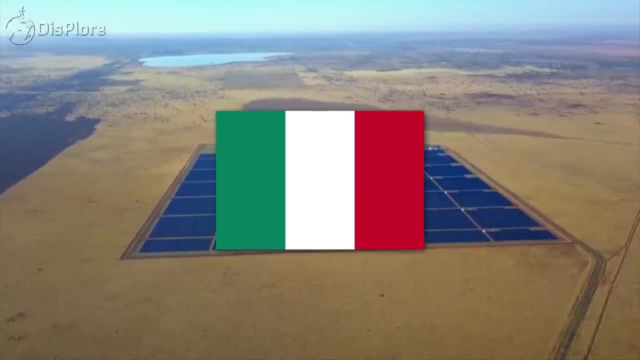 While its chief exports include corn, diamonds, fruits, gold, metals and minerals, sugar and wool, Main trading partners are China, Germany, United States, India, Saudi Arabia and Japan. Others include the United Kingdom, Thailand, Italy and France. 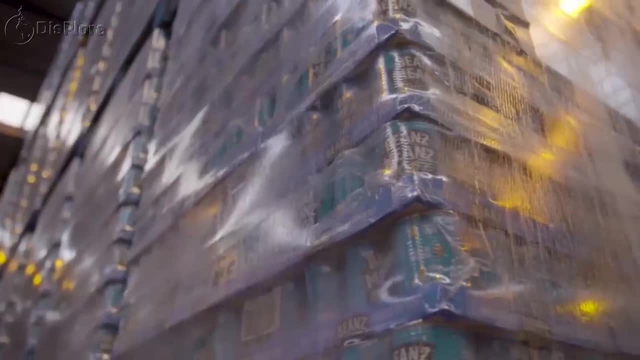 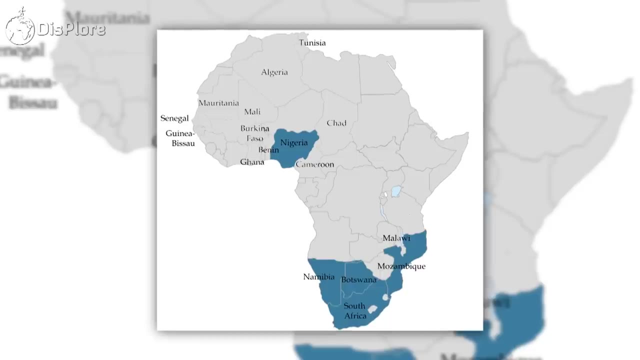 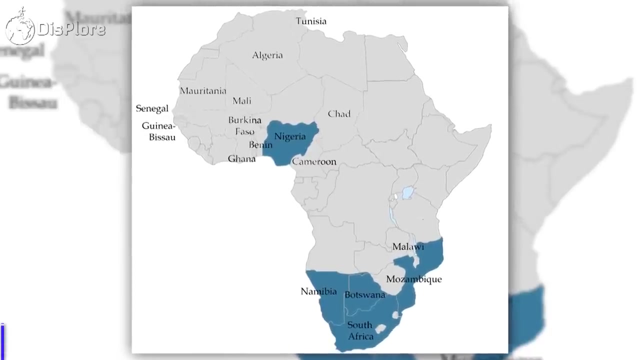 Meanwhile, South African exports to the rest of Africa are predominantly of valid added goods. In terms of South Africa's total trade with the rest of the continent, Namibia, Botswana, Nigeria and Mozambique are South Africa's main African trading partners. 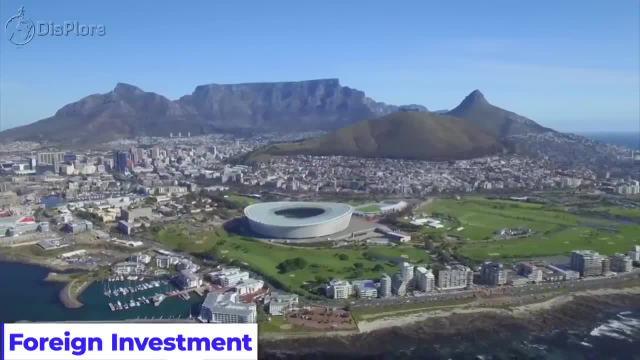 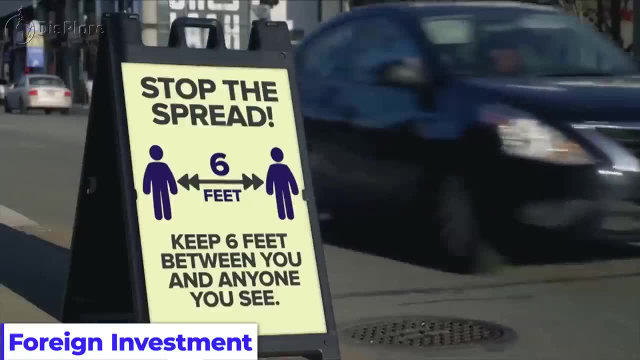 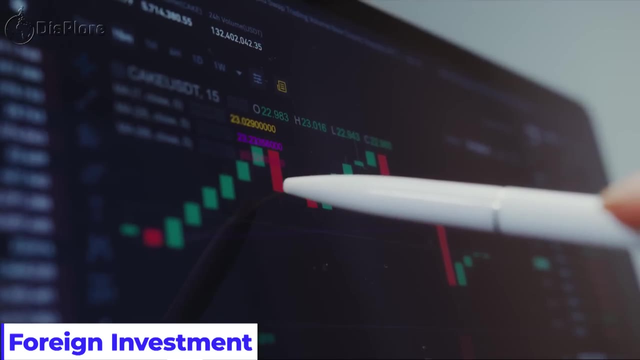 Foreign Investment. South Africa remains the destination for the most foreign direct investment projects in 2022, in spite of the sharp fall in FDI in the continent due to the impact of the COVID-19.. The dynamic business community is highly market-oriented and the driver of economic growth. 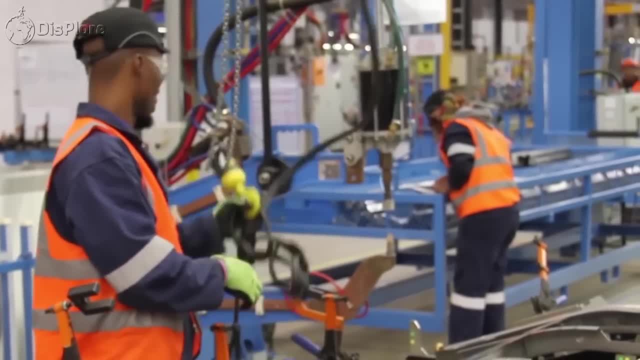 South Africa offers ample opportunities and continues to attract investors. The United States is the largest exporter of oil and gas in the world. It is the largest exporter of oil and gas in the world. It is the largest exporter of oil and gas in the world.